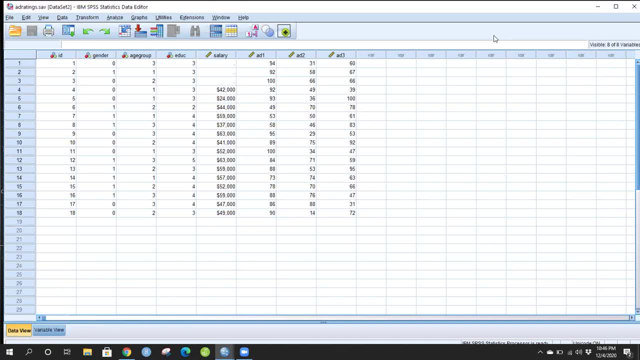 whatever it is, Even if the means are making sense, the sample size is very small, let's say So. we are taking such a case. My sample is of 18 customers, which is a number below 30, and I have data on the gender, age group, their education, their salary. 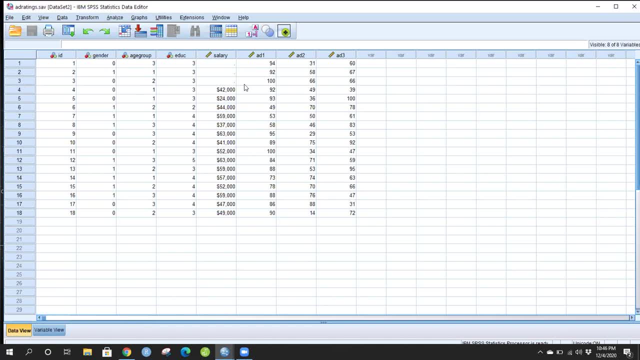 and then I asked those individuals to rate three TV commercials. Okay, so add one, add two and add three are the three TV commercials which these respondents have rated upon, and then we would now be interested in seeing whether these respondents have rated in particularly add one. 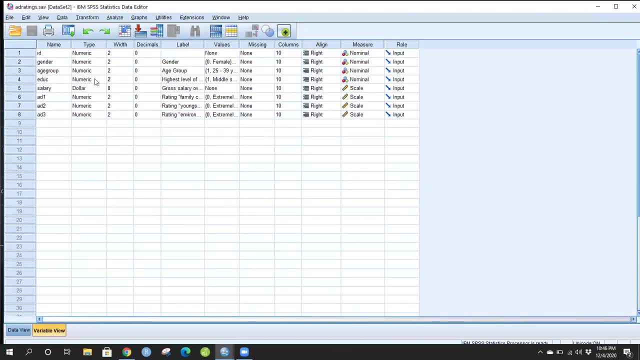 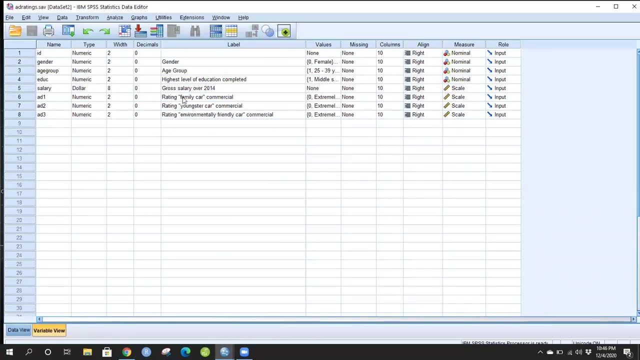 and add two differently. So what are these? add one, add two. So add one is just expand it. So add one is the rating of family car commercial and add two is the rating of youngster car commercial. So it really would be interesting to see that. whether the respondents 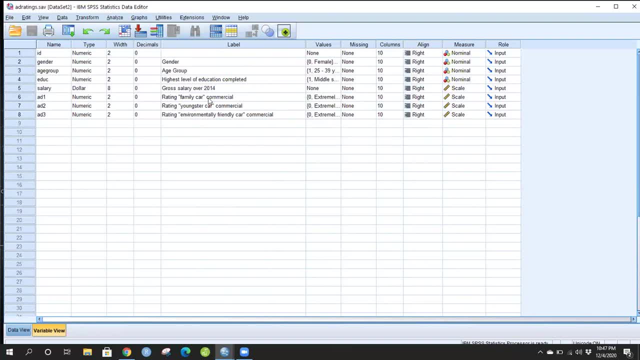 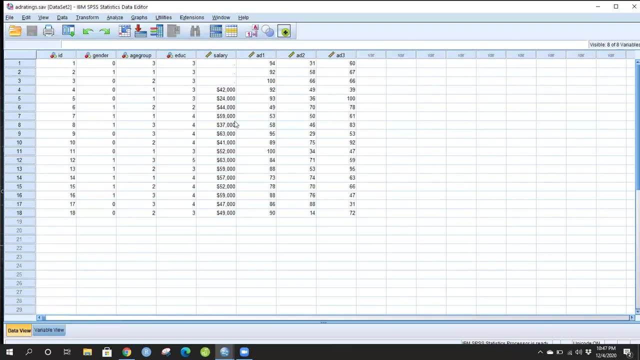 have received family car commercial more welcomingly as against the youngster car commercial, or the either ways. Now, on the face of it, when you compare add one and two, we get a glimpse that the add one rating numbers are clearly larger than add two. Now, because add one numbers are. 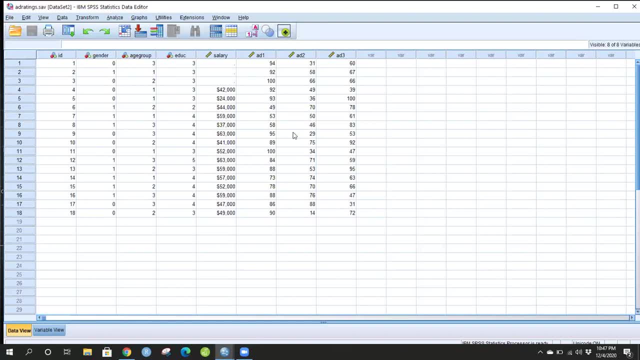 larger than add two. this in a way gives us a hint that probably add one is the variable which is rated more favorably than add two. But can we be so sure about it? We can't be unless we do a statistical test. So here we move on. So Wilcoxon sign rank test is designed for use with repeated 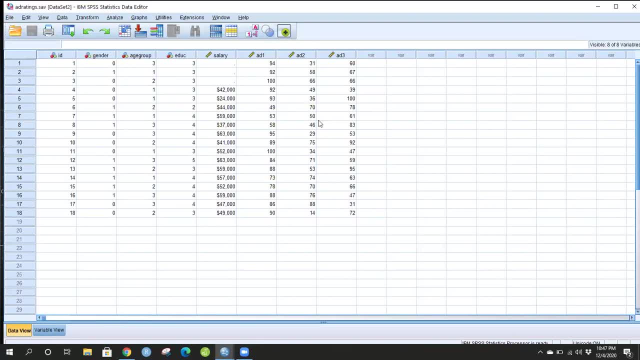 scores, That is, when your participants are measured on, say, two different occasions or under two different conditions, or probably a case like this, when they're really being measured on two different conditions. So one is the condition of add one and one is of add two. And when I said of 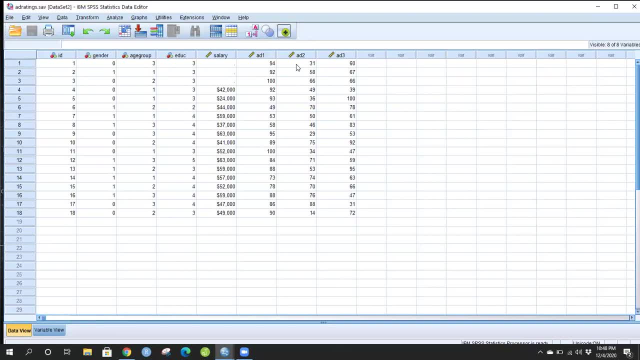 two different conditions. this could also mean that, for example, you are comparing scores on a fear of statistic test administered before and after an intervention designed to help participants cope with it. So that's just an example for you all. Now let's start with this: How? 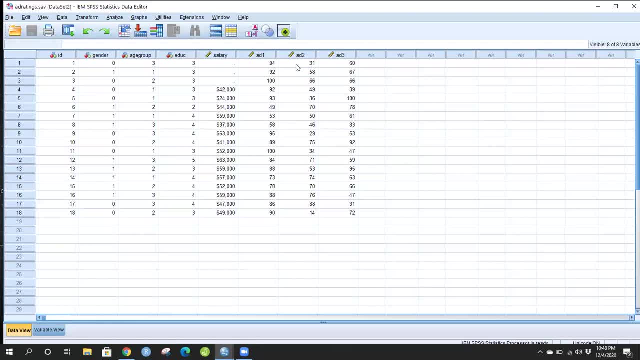 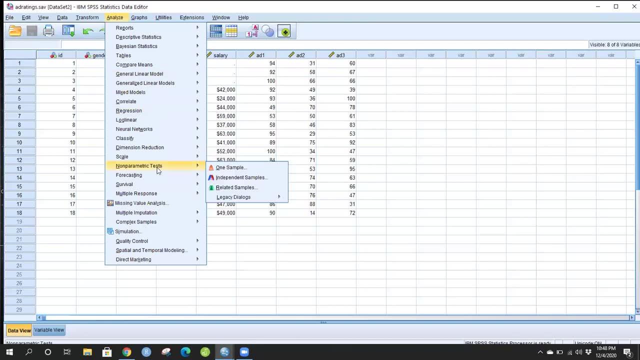 this test really works out? Let's check. So you go to analyze Okay And non-parametric tests, Legacy dialogues, And then two independent- oh sorry, two related samples. So two related samples. So two samples. Can I say that, Yeah, Two related samples Now here in two related samples in variable one and 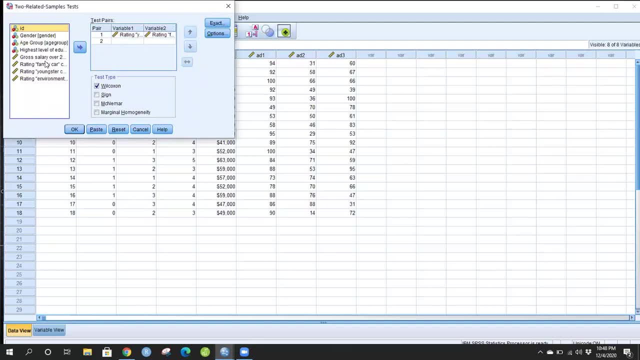 variable two, you have to give you those two variables. So my two variables are add one and add two. So I have passed on both of them And you have to be thought very careful at this stage. This is so because this particular Wilcoxon sign rank test is going to work out by finding out the difference. 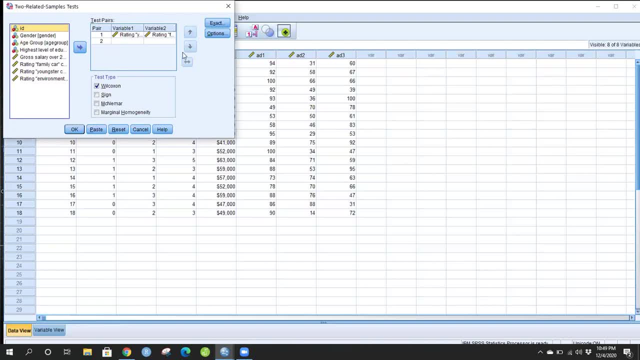 between these two ratings or these two scores, for example. So it's going to be very important to work out a difference between, say, 94 and 31, 92 and 58, 166 and so on. So whenever you're putting variables here in the test pairs, in variable two, it should be the variable with with most of the 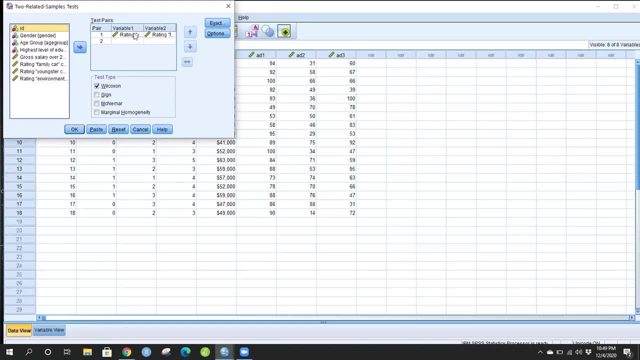 larger scores, Okay, And variable one will be the variable with most of the lesser scores. So in our case, add one at the larger scores, that is, the family car rating. So I have put the family car rating as 55 and youngster car rating as variable one. Okay. So having done that, you go to exact You. 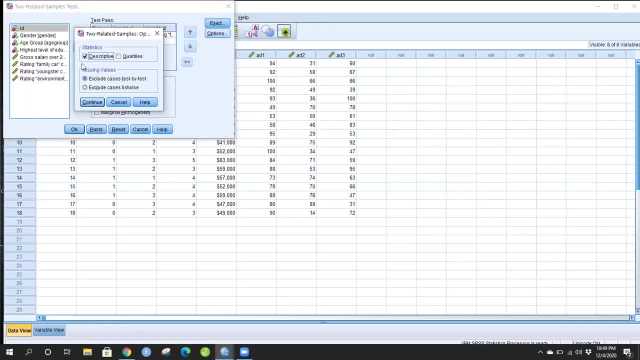 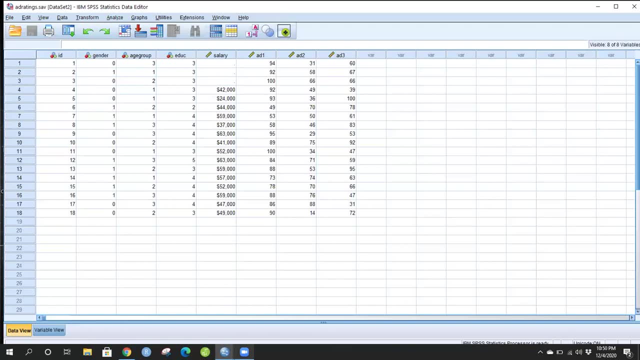 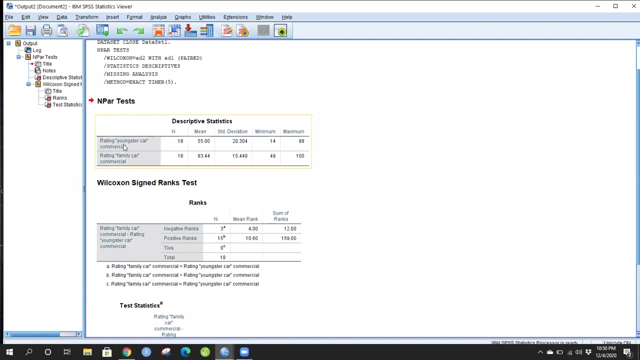 click on five minutes, Then options, Descriptives Continue And test type Wilcoxon. If you click okay, you will have an output like this. So these are the descriptive stats. So the youngster car commercial had a mean rating of 55.. Family car commercial had a mean rating of 55.. So the youngster car commercial 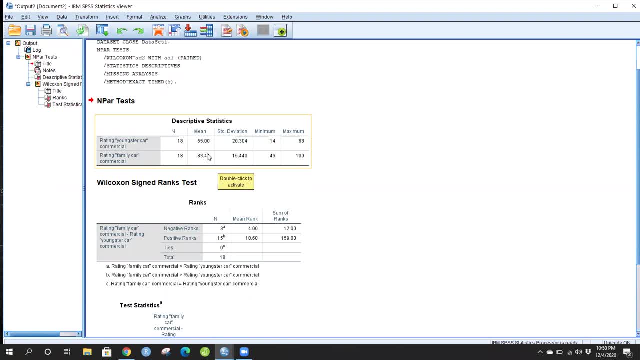 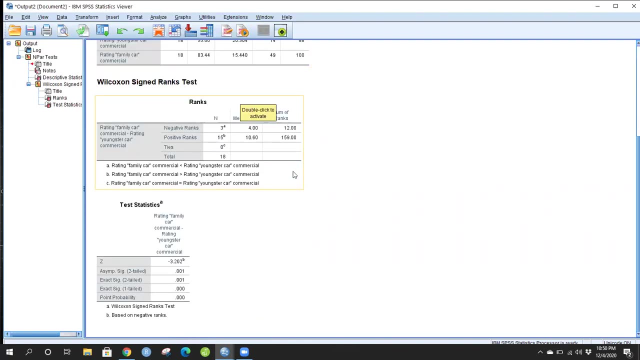 was indeed very well received, with a mean of 83.. And then these are the number of people: 18, 18.. So that that's the sample size usual, The min and max, min and max and the standard deviation. Now this is the table which we must pay a little attention on. As I said, this Wilcoxon sign rank test works. 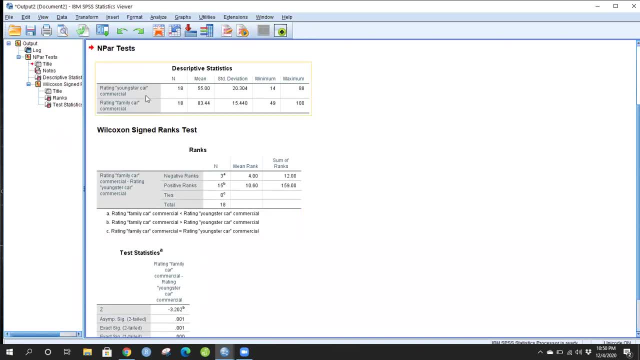 out whether the two variables, youngster car commercial ratings and the family car commercial ratings, are statistically different or not. So the null hypothesis is that the population distributions for both the variables are identical, And alternative is the population distributions for both the variables are not identical. And then, if you are able to reject the null hypothesis, 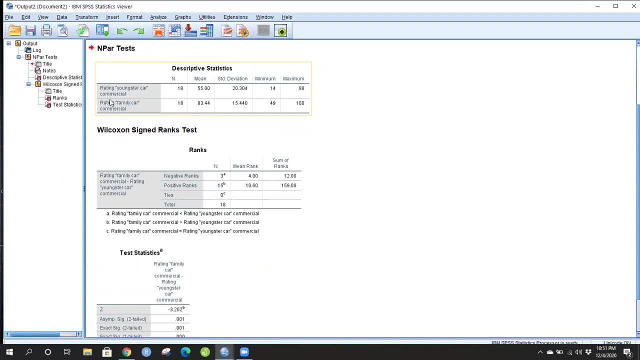 then we can say that either of our ads are rated more favorably than another. So in our case, if we are able to reject the null, we might be able to prove that family car commercial was indeed rated more favorably than the youngster car commercial. 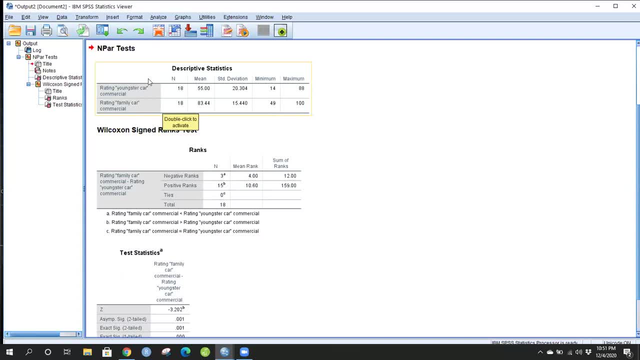 Because obviously family car commercial had higher ratings than the youngster car in most of the cases. So looking at this table of Wilcoxon sign rank test, work this out. So the negative rank, So basically what is exactly? is this finding the? this table is finding the. 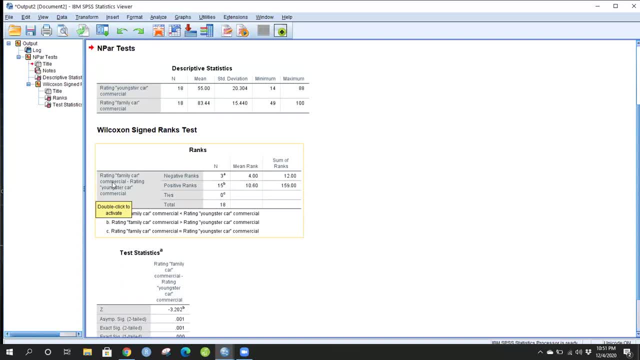 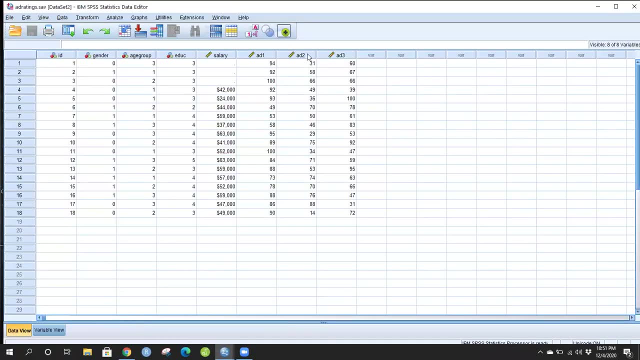 difference. So it calculates the difference between family car commercial rating and youngster car commercial rating. That is as I was explaining you with the example. So it is going to work out these differences: 94 minus 31, 92 minus 58 and 73 minus 34 and so on. 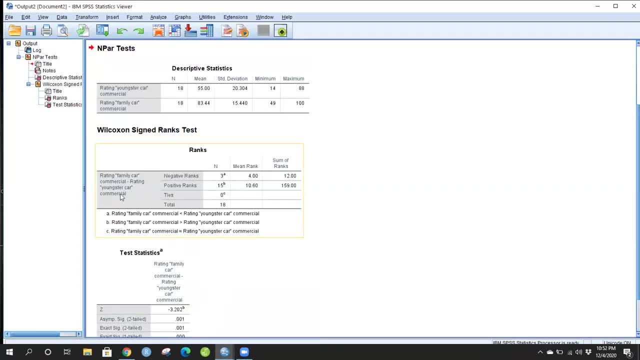 So all these differences will be worked out and then it will tell that in how many cases was a negative rank observed. that means the difference worked out to be negative. What does a negative difference mean? negative difference would obviously mean that youngster car commercial was rated higher. 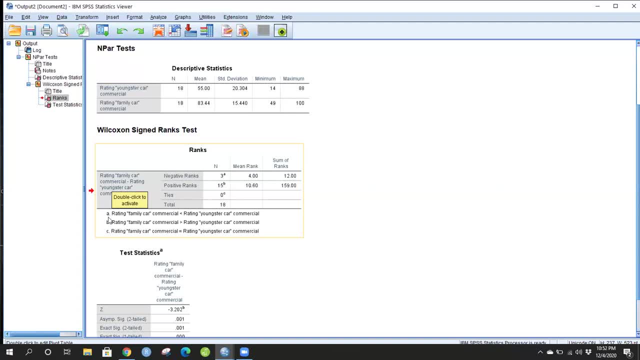 then only the difference would be negative, right? So they've also written it here and as a the superscript is explained here that if you have a negative rank, That means the family car commercial rating is lower than the youngster car commercial rating, and if you have a positive rank, then the youngster car commercial rating is lower than the youth car commercial rating. 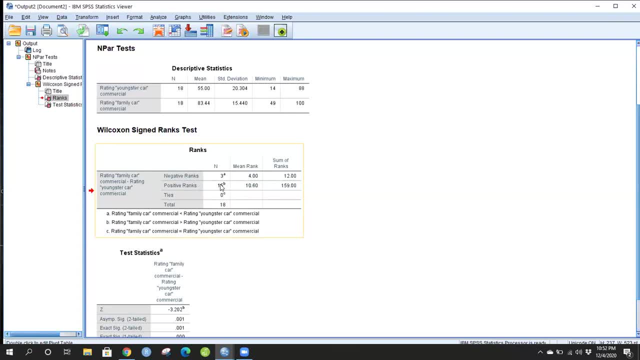 And if you have a positive rank, and we have 15 such cases of positive rank. so out of the total 18 cases, three cases are with negative ranks and 15 are with positive ranks. so positive ranks mean that rating a family car commercial was higher than rating of the youngster car commercial. then this is the mean rank. so in 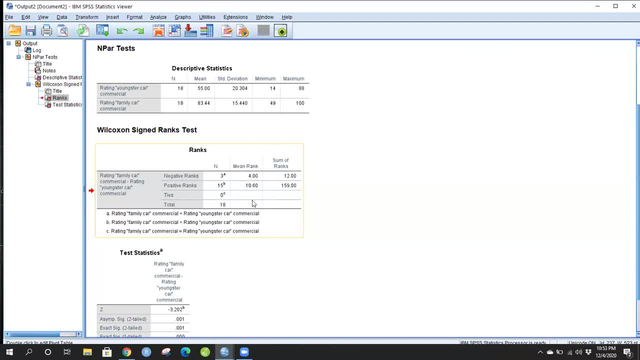 the negative ranks. what is the mean in the positive ranks, what was the mean? and then these: this is the sum of all the negative ranks and this is the sum of all positive ranks. okay, actually this works out with absolute differences, so you need not bother about the calculations a lot. 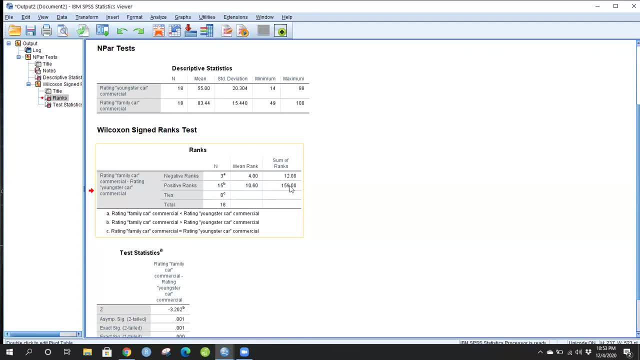 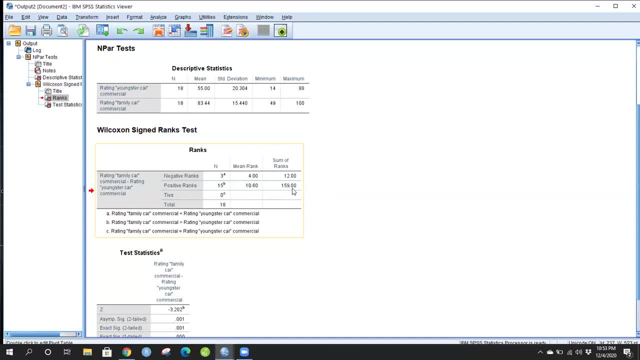 very small or very large. if it is, then that is indicative of different distributions of both of these variables. if it is either very small or very large, that would indicate that these two variables are indeed coming from different distributions. so, finally, we see that this number is, come, you know, a very large number. but right by looking at this number, we cannot say that. 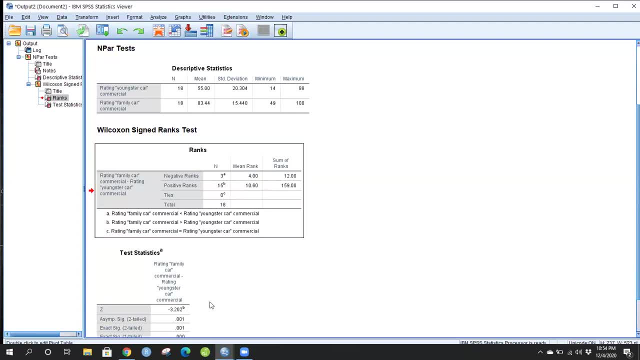 the statistics has changed, so we can't say that the statistics has changed. so we can't say that. we can't say that ones multiplied by four, unfiltered ones multiplied by 4. so what we can do is actually do, is actually do this, so you get, you get this number from you. know the one thing. 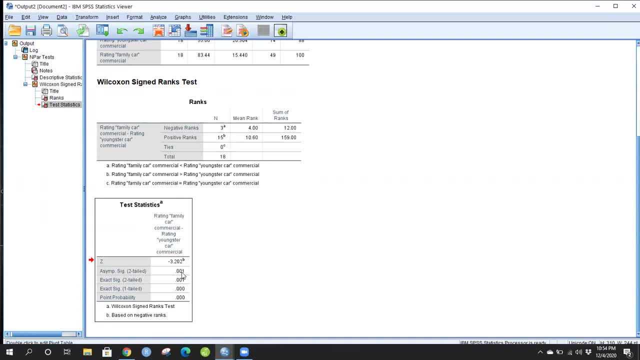 we can do is just actually check whether your total numbers are positive or the same. this is the assumption here. is that so we can say whatever number it is really, its name is positive degree. how often can you study it? no, we can actually change the value of this and let's say it is. 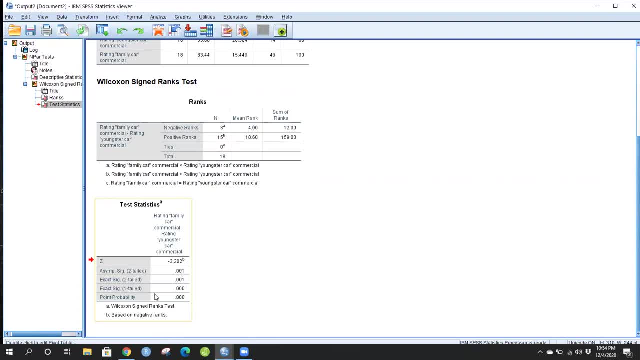 just not working for us and our way of Mechanistic colonies is just to say I need a definition of these two. we can look at all the known rankings: sting null hypothesis of population distributions being identical gets rejected. So in our case, as we show, as we have shown that the sum of positive ranks is way larger than the sum of negative ranks. 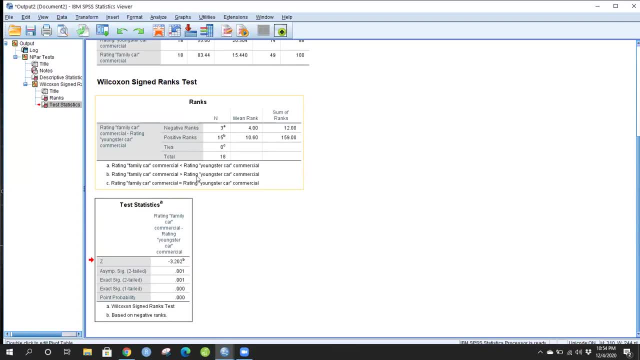 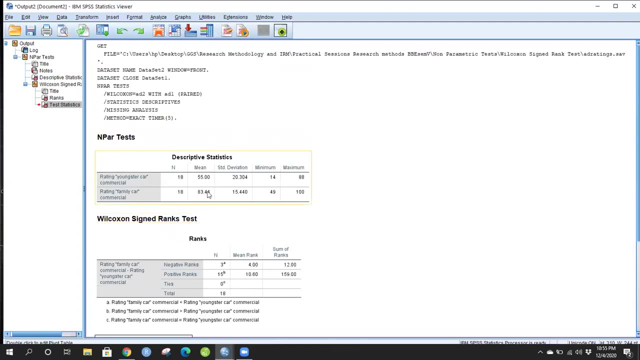 which was giving us an indication that family car commercial is rated higher than youngster car commercial, is now proven statistically also. So we can say that the Wilcoxon sign rank test has indicated that the family car commercial, which has a mean of 83.44 and was rated more.